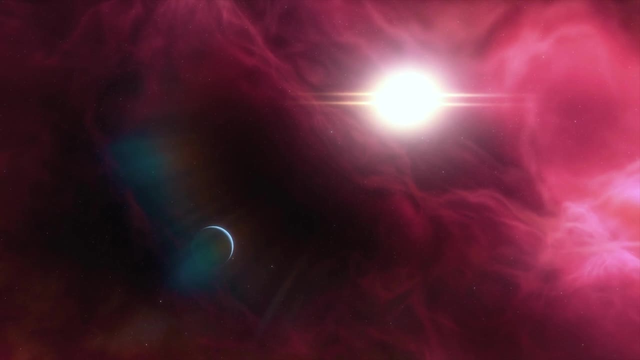 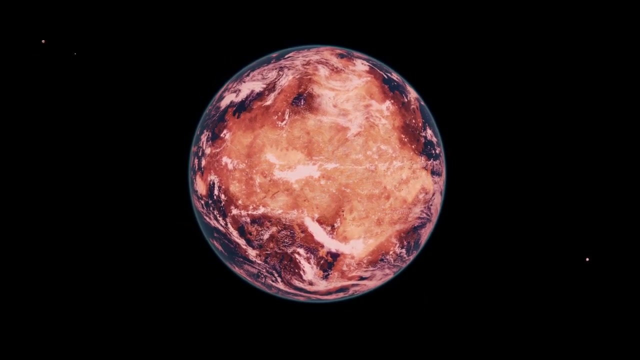 Astrometry is the most ancient method of searching for extrasolar planets. As early as 1943, astronomer Kai Strand of Swarthmore College's Sproul Observatory announced that his astrometric measurements revealed the presence of a planet orbiting the star 61. 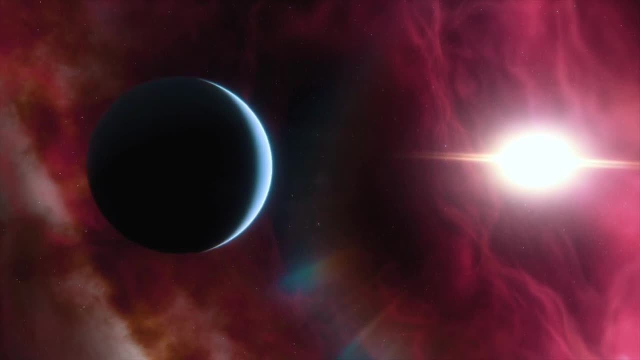 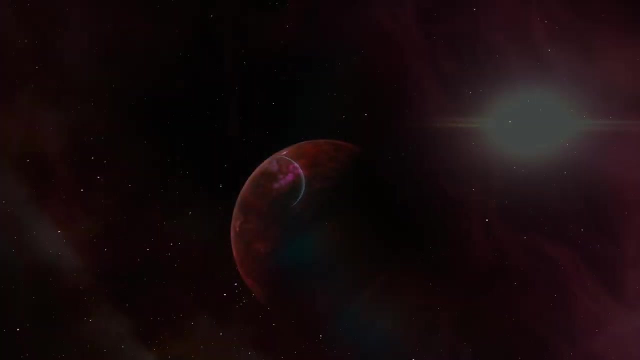 Cygni. Astrometry is the precise measurement of a star's position and movement. When planet hunters use astrometry, they use the method of searching for extrasolar planets. Astrometry is the most recent method of searching for extrasolar planets. They look for a minute. 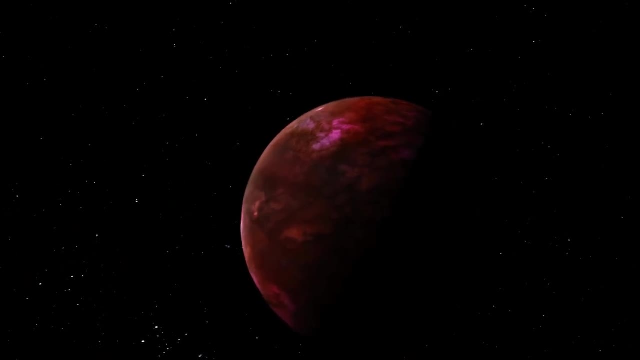 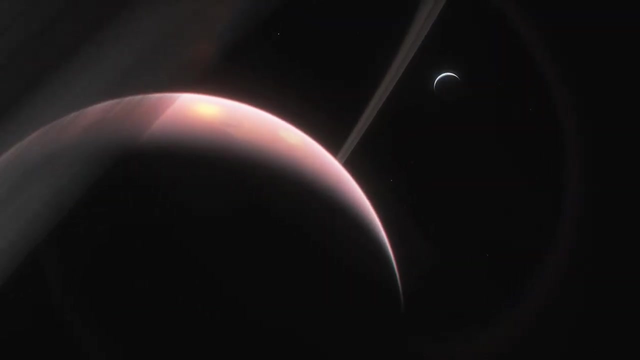 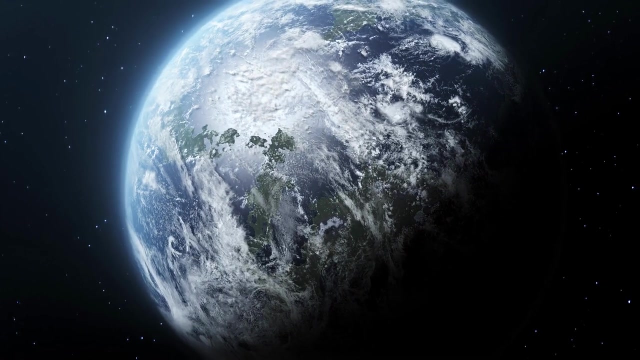 but consistent wobble in a star's position relative to other stars. If a periodic shift of this magnitude is detected, it is almost certain that the star is being orbited by an unseen companion planet. Astrometry is one of the most sensitive techniques for finding 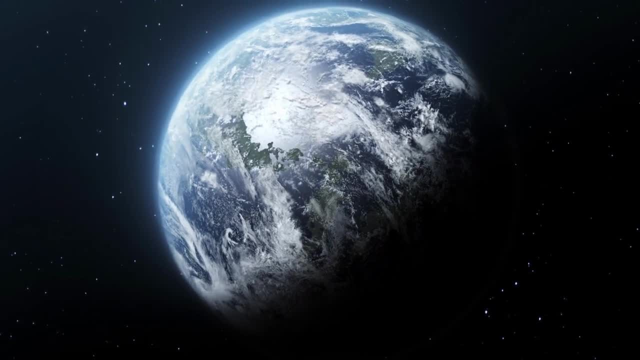 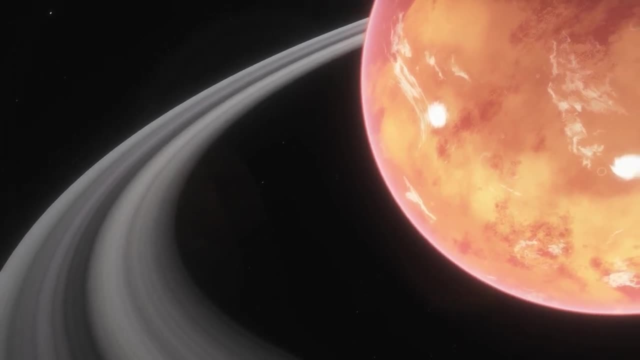 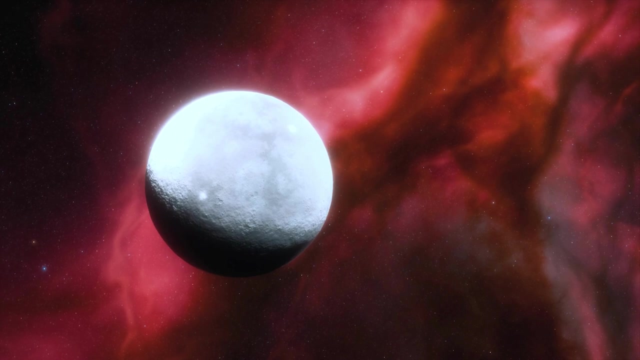 extrasolar planets. Astrometry can be used on a much larger variety of stars because, unlike transit, it is not reliant on the distant planet being in nearly perfect alignment with the line of sight from Earth. Astrometry also provides an accurate estimate of a planet's mass. 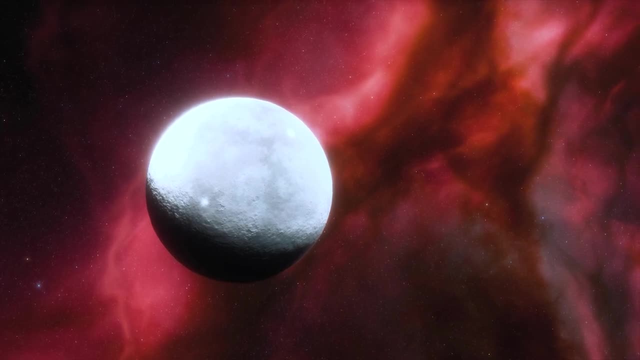 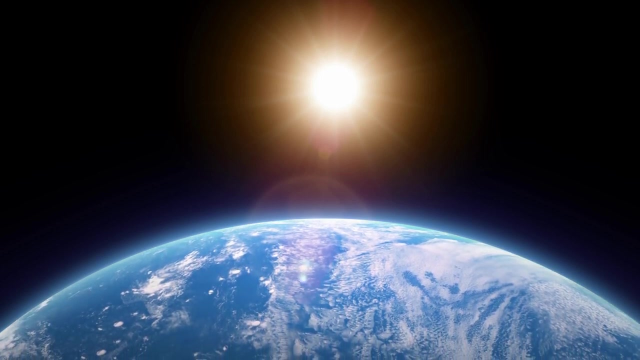 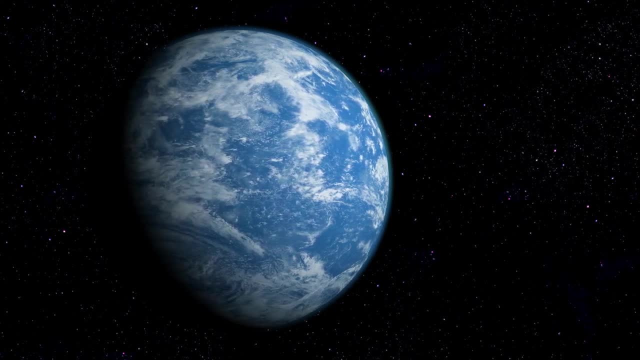 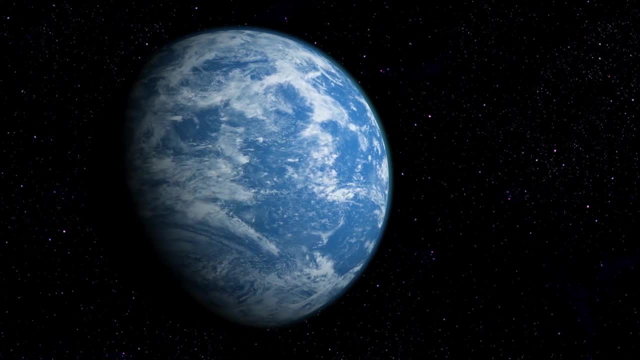 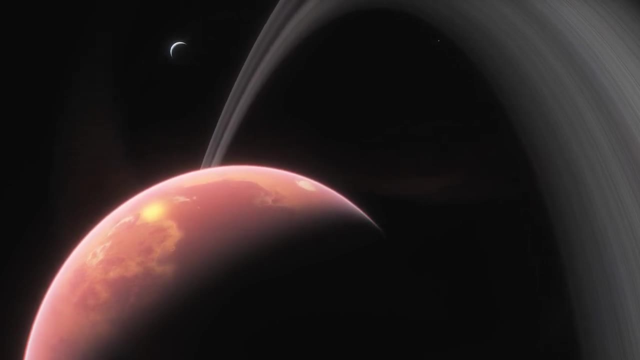 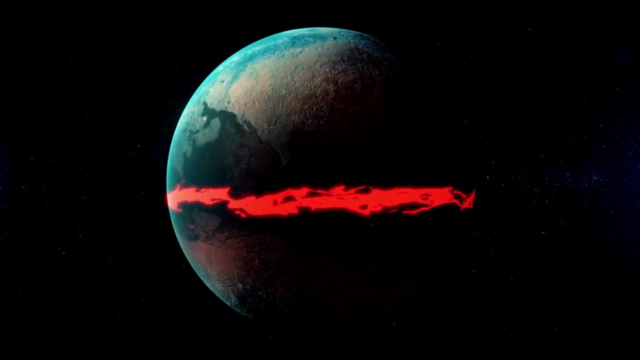 even with the largest and most advanced telescopes, This method is not great for determining the exoplanet's diameter and it is very difficult to detect many exoplanets at once. Using another method like spectroscopy, in parallel to astrometry, may make it easier to detect exoplanets with 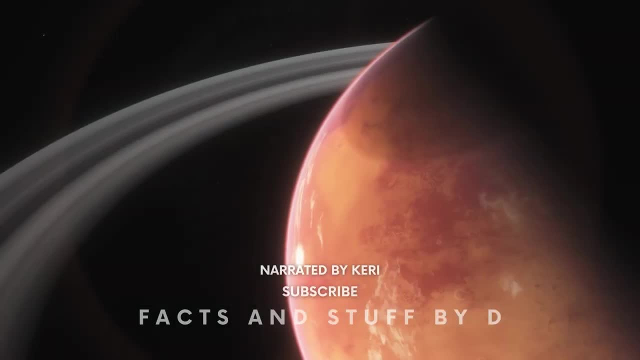 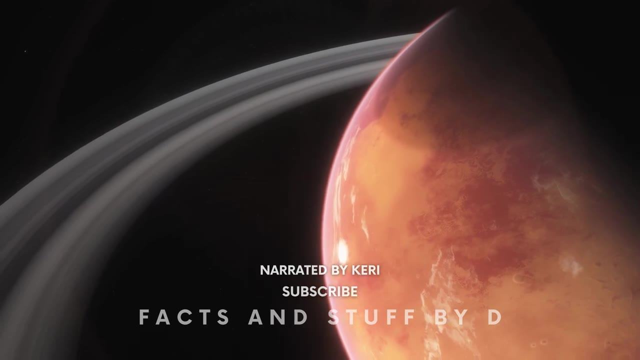 greater accuracy and precision. Thank you for watching and please subscribe to the channel.